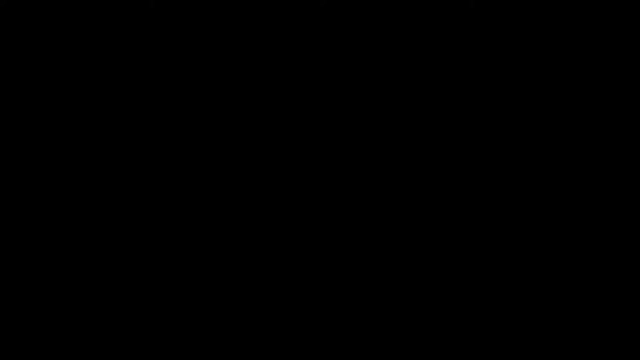 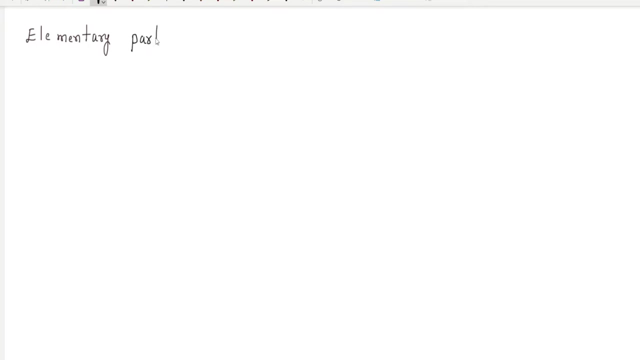 Thank you. Thank you. In competitive examinations they are giving one reaction. Try to ask what type of interaction takes place in reaction: The gravitational reaction or the electromagnetic reaction? or a weak interaction or strong interaction? So for that we need to know what type of interactions are there in between the 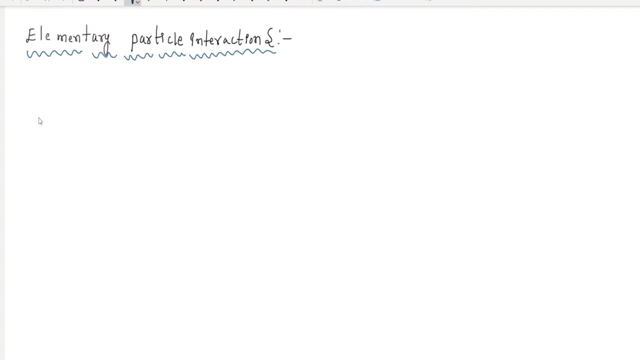 elementary particles. The interactions among the elementary particles give information about various properties under decay modes of the elementary particles. So there are four types of interactions among elementary particles. One is a gravitational interaction. Second one is electromagnetic interaction. Third one is strong interaction. 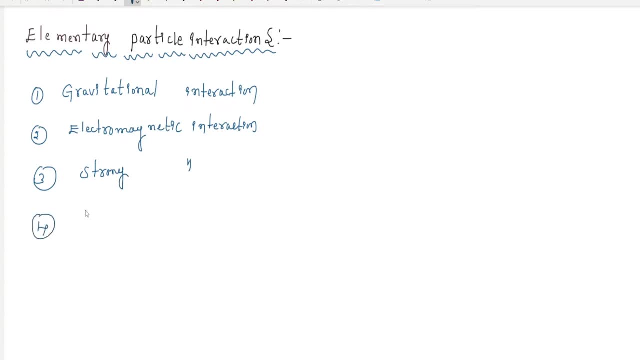 Fourth one is weak interaction, The gravitational interaction. in order to understand the gravitational interaction, so we know Newton's law of gravitation: F equal to F equal to g, m1, m2 divided by r, square right, If the m1 and m2 are markers of the object, r is the distance between the particles. 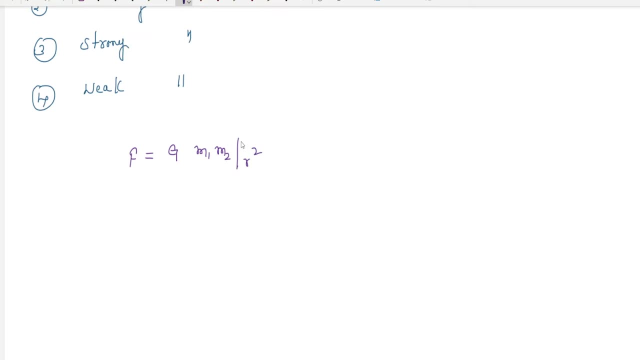 g is the gravitational constant. The gravitational force does not depends upon the color, size, charge, velocity and the spin, So these are important, But it depends on magnitude of momentum of energy. In case, if you try to calculate this, you get the following linearly kinetics: 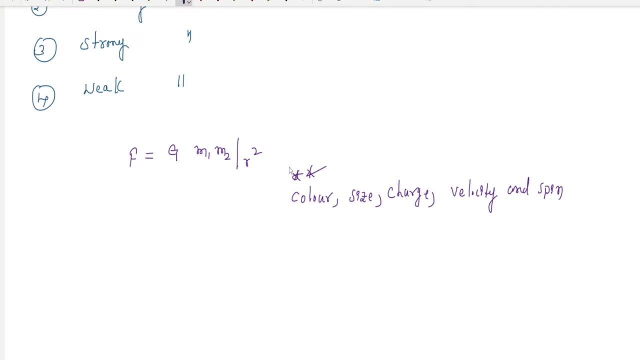 Calculate. the gravitational force between the two nucleons is roughly 2 into 10 to the power of minus 34 newtons. This is one letter And other case. the gravitational between neutrons and the gravitational attraction is about 2 into 10 to the power of minus 49 joules. 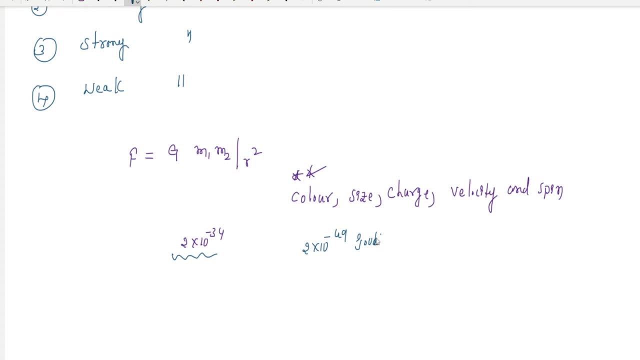 Okay, So hence the gravitational attraction among the elementary particles is very weak and negligent, right? So in elementary particles the gravitational force can be explained in terms of interaction of gravitants. So we know, the gravitants belongs to the bosons categories. 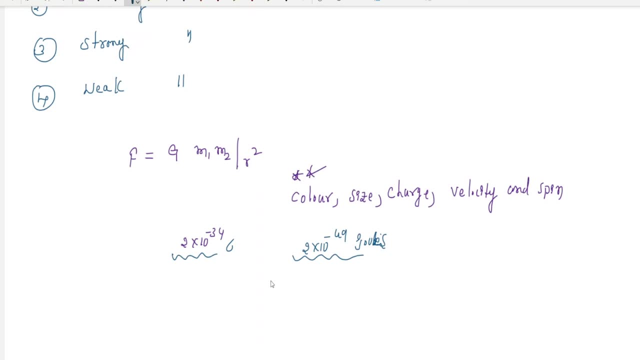 Since these particles are the massless bosons and travel with the speed of light and the gravitational field is very weak, the gravitants cannot be detected in laboratory. So this is all about gravitational field. Next, in case of elementary particles, 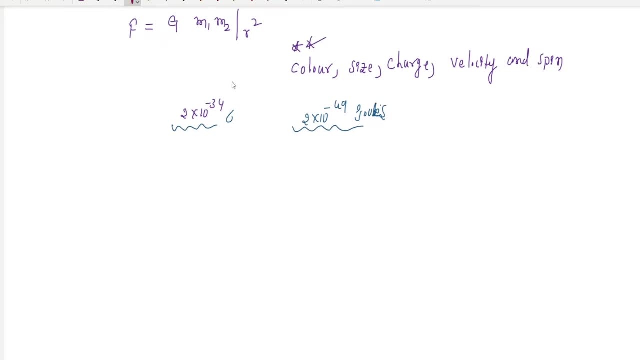 So in case of electromagnetic interaction, in case if you try to know the EM interaction, EM interactions, the electromagnetic interaction can be explained by the Coulomb's law. We know that this Coulomb's law F is equal to Q1 and Q2 divided by 4 pi. epsilon naught half square. 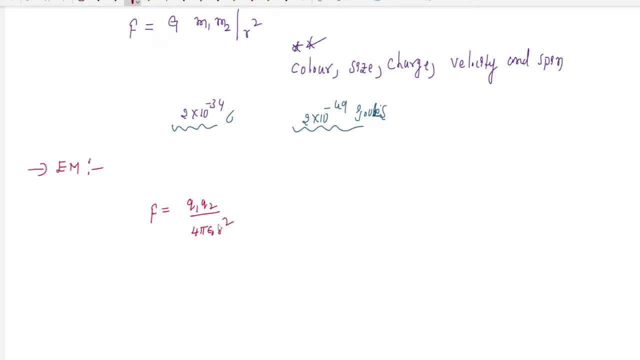 Q is charge, R is the distance between the particles. Electromagnetic forces operate on charged particles and provide atomic binding forces. right, The electromagnetic forces mainly depends on the discharge. If you calculate the electromagnetic force between the two elementary particles, it is around the roughly the 30 Newtons. 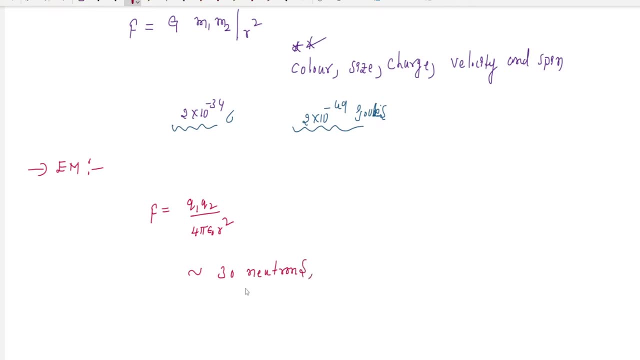 So the emi force is almost 10 to the power of 35 times greater than the gravitational force. the strong, i mean the strength of electromagnetic interaction is given by the dimensions uses the fine structure, constant, alpha right. so we know already alpha, fine structure, constant alpha equal to e square divided by 4 pi, epsilon naught. 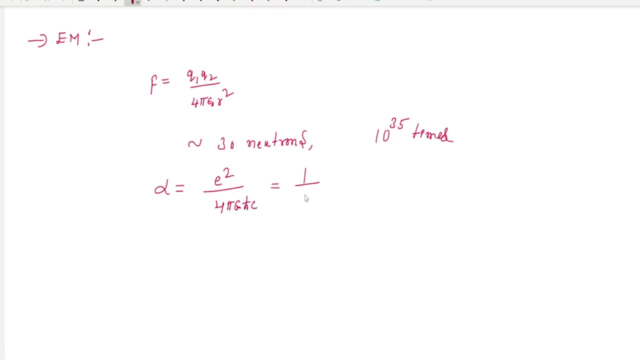 h cross c right. so this is almost 1 divided by 1, 3, 7.. this is the key point here. the, the em interaction is mainly due to the exchange of field particles, photon. so example of this uh electromagnetic interaction is the bates formation and the decay of mesons. 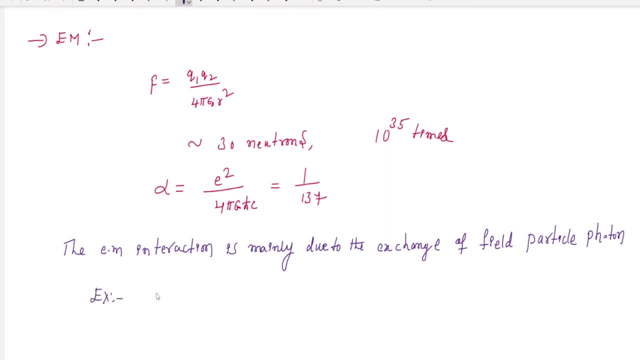 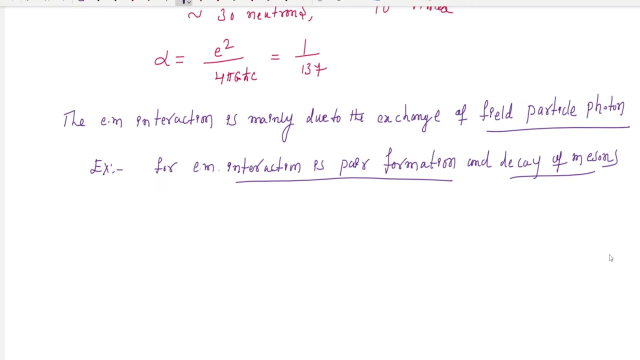 d�, tr, it is. i use b i to in came by using this point. we can make some shortcuts and we can problems easily. mesons- the word is very important- by formation: neutron field, particles, photon. okay, next, strong interaction. uh, strong interactions are responsible for holding nucleons together even if the strong repulsive force exists between. 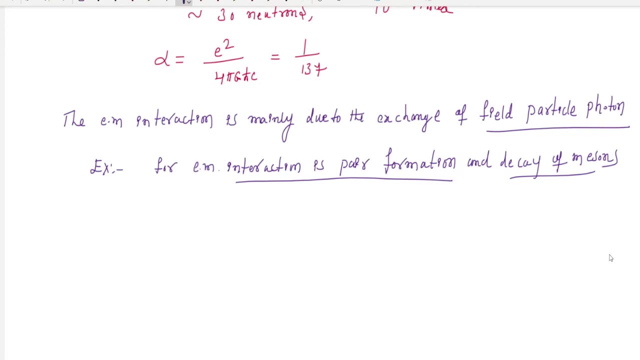 them. this force is depend on the electric charge and cannot be expressed in terms of strength, distance relations. this force is very short range order force. almost a strong interaction is a short range order force, strong interaction. so short range of the order 10 to the power of minus 13 centimeter. 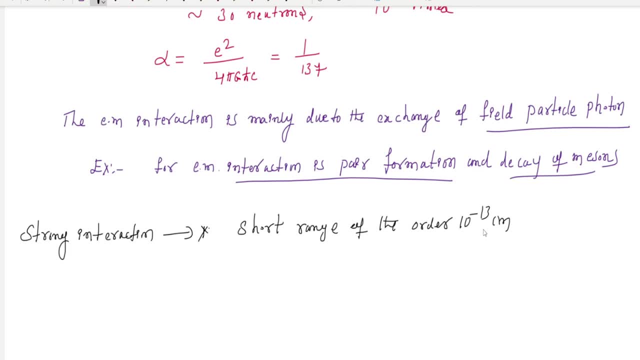 the time travel of a strong interaction is, uh, almost 10 to the power of minus 23. second, the strength of strong interaction is given by the this formula: g squared divided by 4, pi, h, c, equal to 100, into alpha: okay, this strength is 10 to the power of 3 times. 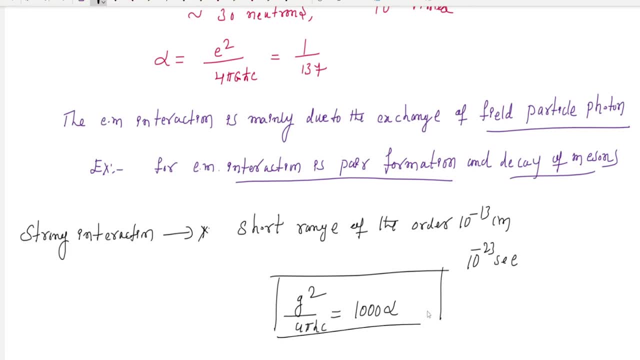 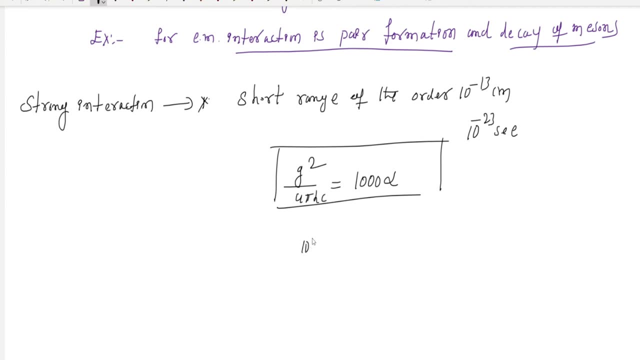 greater than the image term: okay. so 10 to the power of 3 times greater. greater than 3 times greater than the image term okay. example: this is strong interaction: scattering of mesons, nucleons by nucleons. so examples: scattering of mesons, nucleons by. 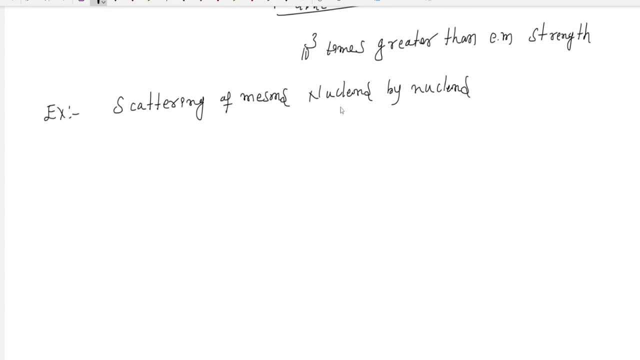 nucleons. okay, next, weak interaction. we know that the characteristic time of the strength interaction is 10 to the power of minus 3 seconds. when these are just now, we discuss about strong interaction between the weight of nucleus right immediately faster t under the power of minus 23 seconds. something new: particles may be produced. 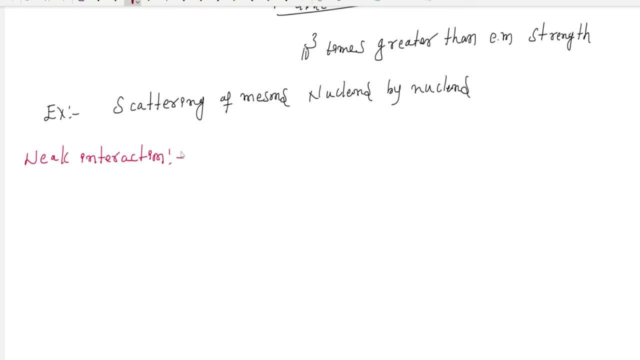 some new particles. but it is observed that the product of new particles- uh, maybe decay mode or formula, only after 10, to the power of 10 seconds and the power of minus 10 seconds. so this is first explained by the 1930- used N weighing AHCO N traverse on. this is first explained by the 1930. let me explain that some. 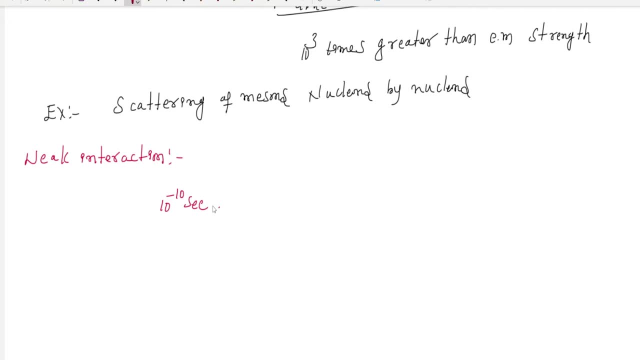 금 gramikum and the across material third cell reduced resistance that some particles takes long time to highly tinha 're going to know the acompan his or unplug his cell. so some of them are not there such process. So the force involved must be weak compared to the strong interactions. 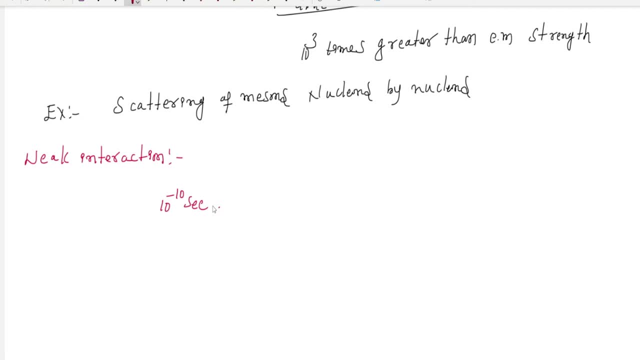 as the term becomes to weak interaction. So best example is weak interaction is a beta decay from the radioactivity. So from this, all the theoretical description, I am going to make some shortcuts. Okay, How to identify whether the interaction is strong or weak? 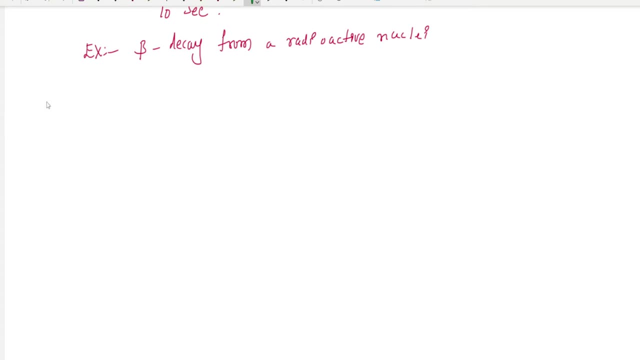 Okay, There is no gravitational interaction. We can neglect gravitational interaction. electromagnetic interaction, the weak interaction. So three type of interactions are there Here. I am going to make one table. This is charge, This is lepto number, This is barrier number. 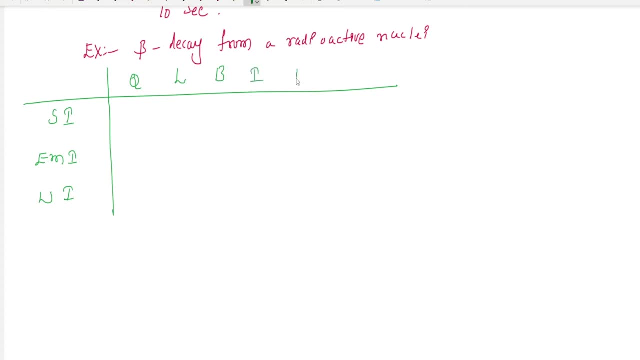 And isospin also there. Okay, I3, and this is strenuous number. Right In case the given reaction is: follow the charge: lepto number, barrier number, isospin, third component, strenuous, Then that is the type of reaction. 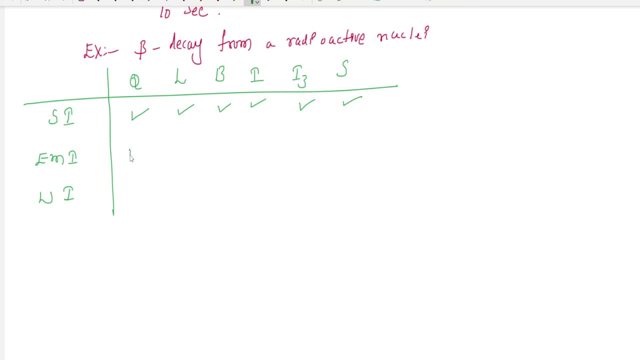 This is strong interaction In case of electromagnetic interaction. so charge is Ronendealt, lepto number is Konzel, barrier number is Konzel And and maybe isospin is not Konzel, I3 is Konzel, so this is also Ininoskeletal. 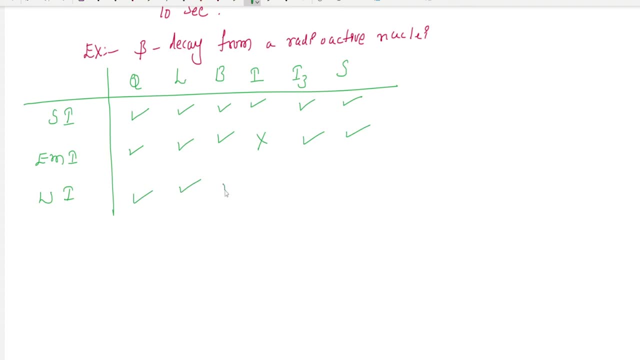 This is also Konzel. Weak interaction is Konzel? Lepton number is Konzel? barrier number is Konzel? Maybe this is not. This is also not. This is how we can check the- either a weak or strong interaction. okay, so the here i'm going to make one note. uh, do one more. okay. so important keynotes: weak interaction. 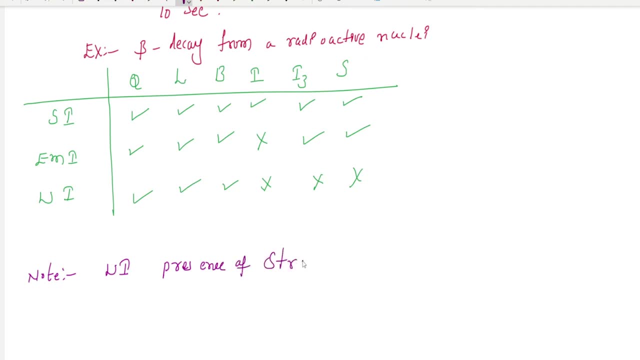 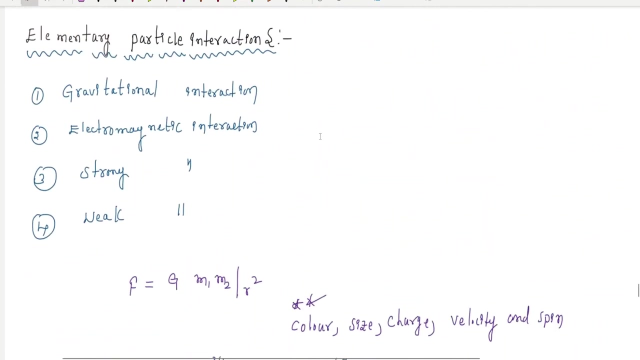 presence of strong particles. okay, for example, delta is equal to plus or minus one. this is strong interaction. strong, for example, delta s is equal to zero. this is may be a weak interaction. so from this uh description what we discussed- gravitational, electromagnetic strong interaction, weak interaction- we can make some key points from. 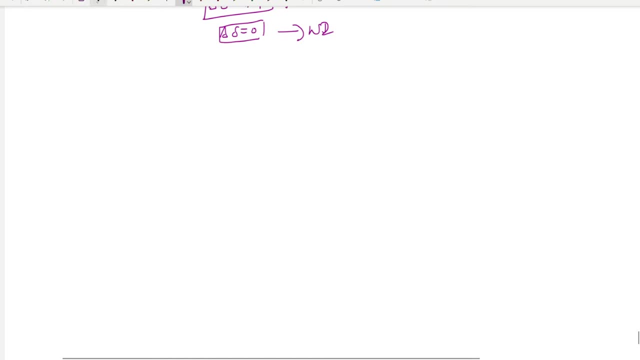 their description points. so wrong interaction is a wrong interaction. electromagnetic interaction, weak interaction. so here the first point i'm going to tell you: these are all head runs. there are shortcuts in case in reaction present. all head runs. that is interaction. this is one key point. second key point is associate productions. group of strong particles. okay, 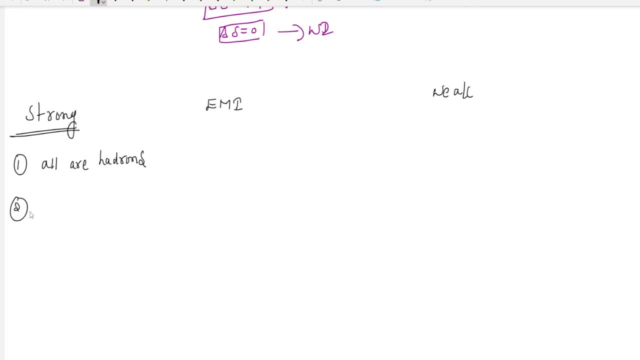 group of strong particles. so, and no lepton present in that reactions. remember these words. okay, this is a shortcut. next, em interaction. first keynotes, in case, if photon- we already discussed this thing- present. so you know photon, right, that is your main traction particles and its anti-particles. 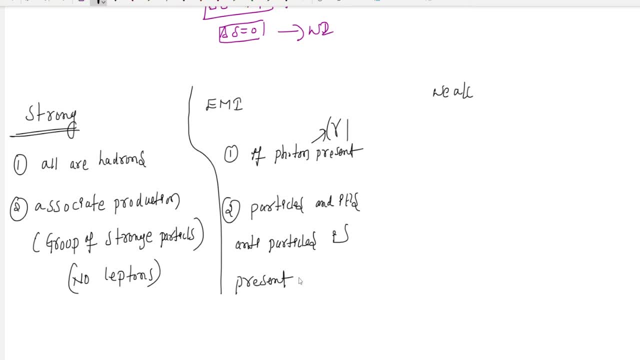 is present on one side of the. so these are all shortcuts. okay, it has come to weak interaction. first bullet point: is any one laptop present? second bullet point: strong particle decay. so s particle decay. strong particle decay example: very strong person. okay, this type of particle stick. now it is time to check. uh, previously your question here. i'm going to check quickly. 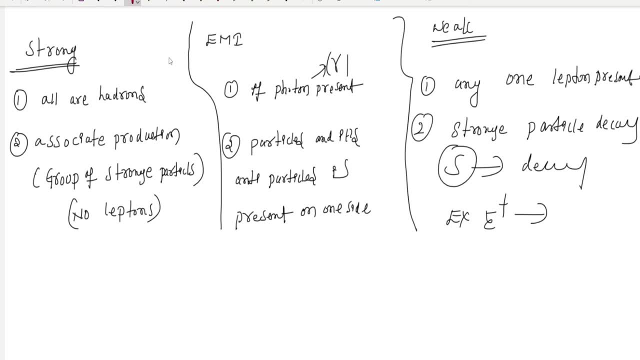 three reaction number one: okay, first equation i naught tends to photon plus foot. what type of reaction is one if photon present? that is just two seconds. within two seconds you can get the answer shortcut form or else we need to remember all these points. whatever we discussed here is right. some. 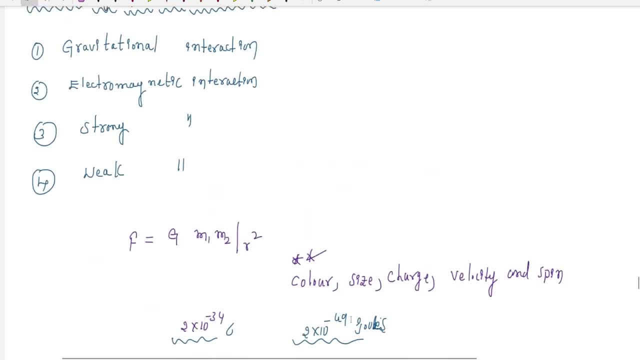 key points we discussed here. so it is depends on results, not even some examples. we need to remember all this effect and make the note like: like this, then you can be able to do it. okay, so we can keep should probably from what else are dreamer, and before after unlock, then we need to remember this. 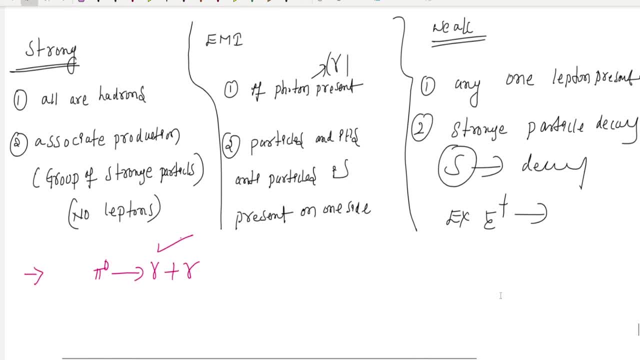 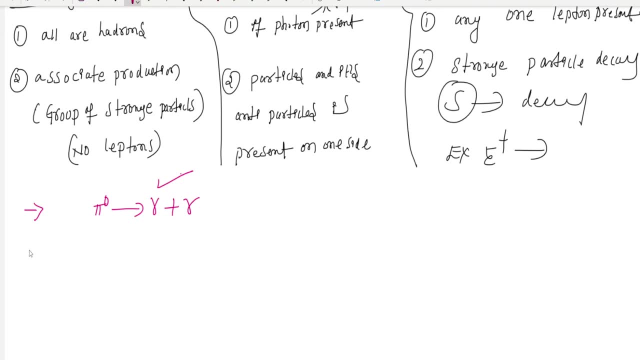 like, like this, then you can go along with this. so in complete exams not only depends upon the derivation, not subject important, but also it is very important to learn. shortcut tricks doesn't mean you shortcuts always works in international exams. so 90%: you need to focus on the concept: wise problem. 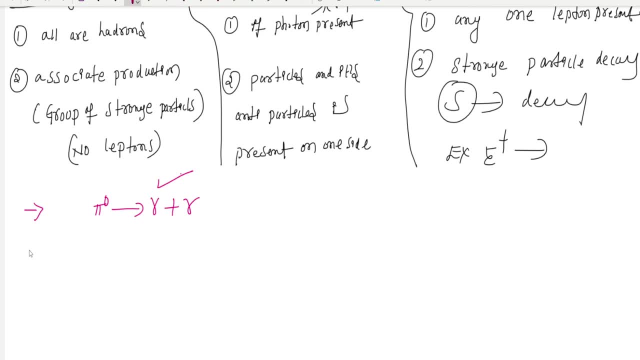 solution. then you can understand better, then you can make your own shortcuts by observing this question. framing all this in next question: K minus photon: a place less is strong part. okay, what type of interaction takes place here? on type of interaction, add-ons are two, two, two, two. 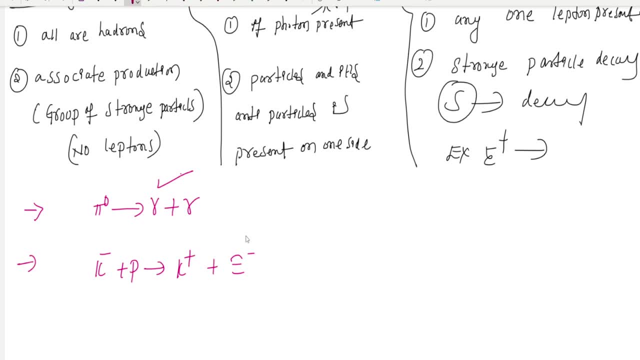 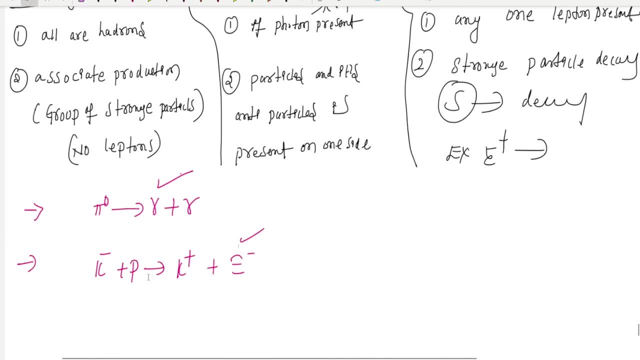 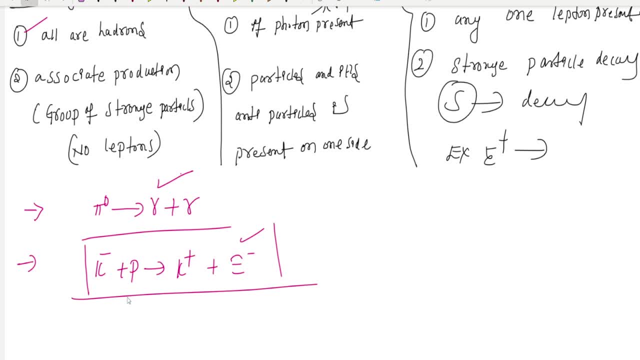 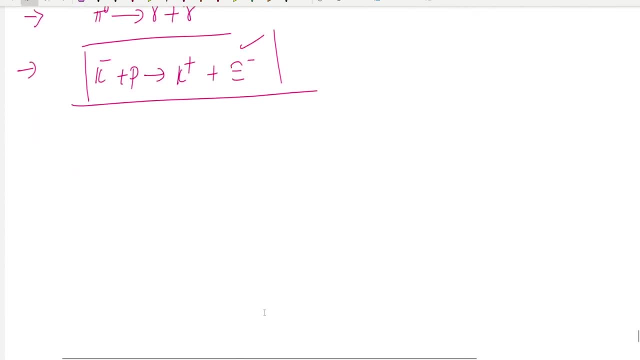 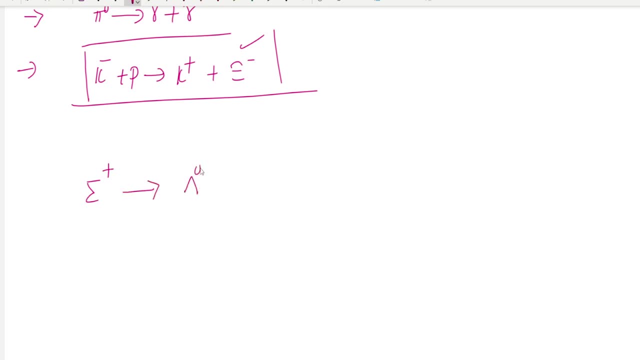 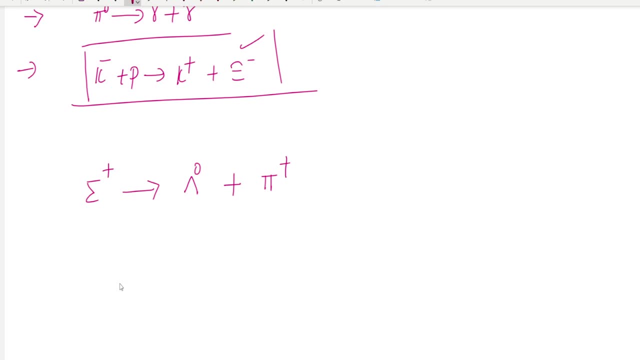 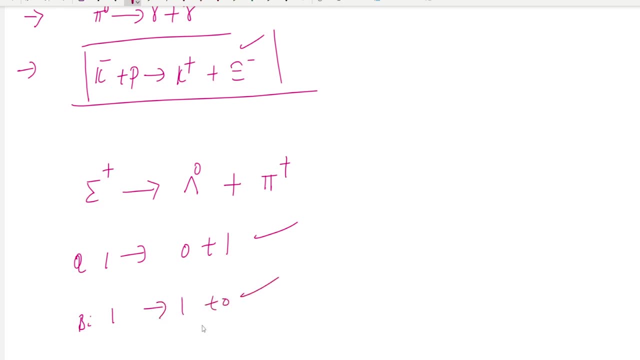 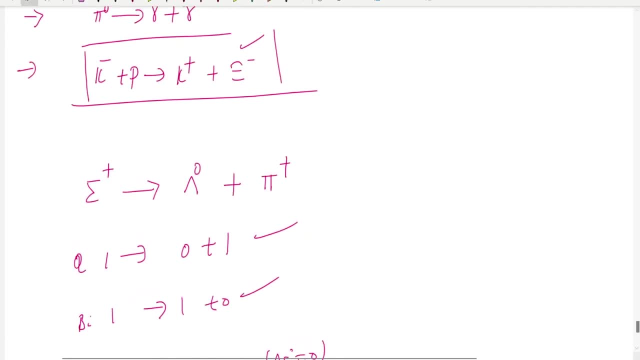 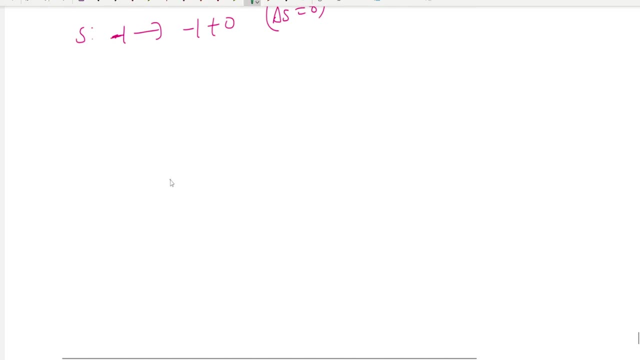